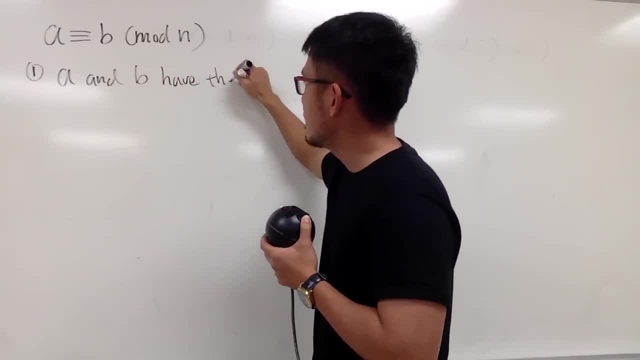 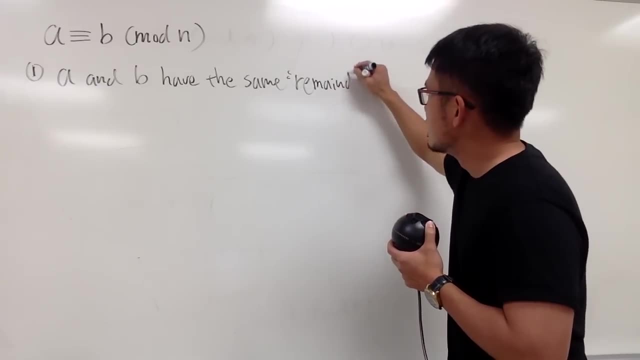 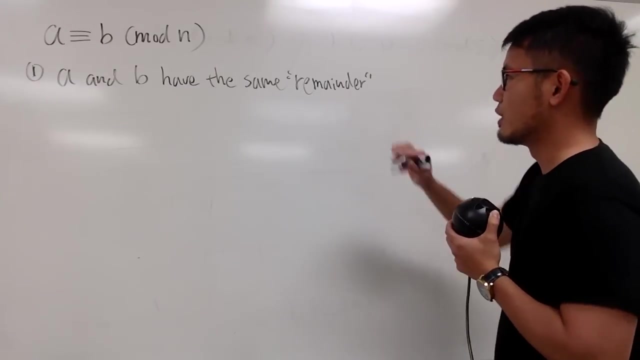 and b have the same remainder and i will put on quotation mark for the word remainder because sometimes when we're talking about this kind of things, you may enter with negative reminders and things like that. so that's pretty much idea. that's why i put down quotation mark. 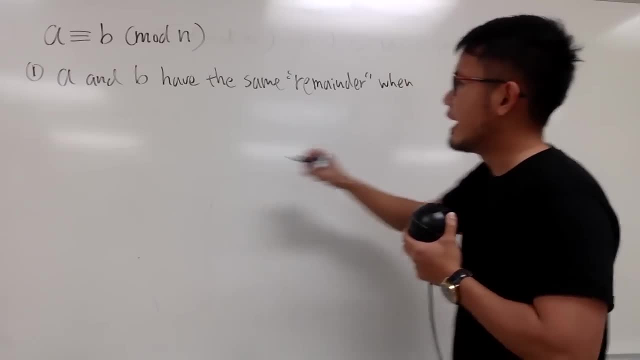 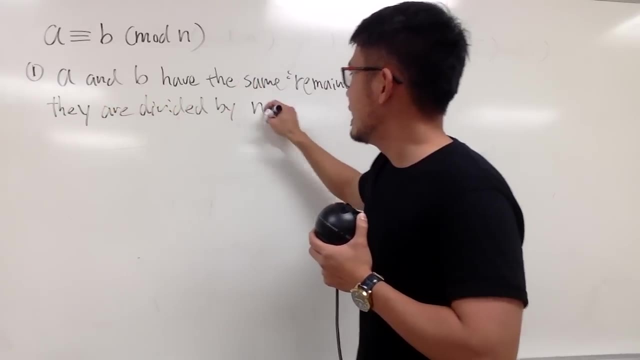 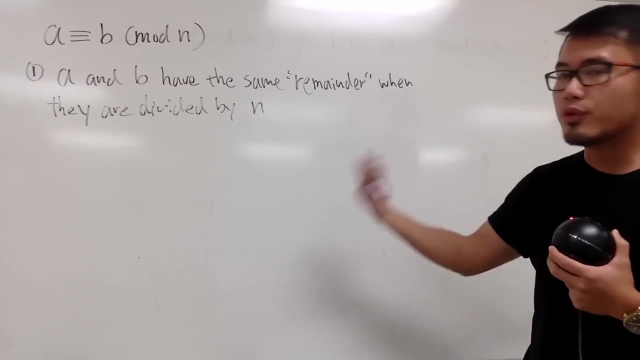 a and b have the same remainder when they are divided by n. okay, and by the way, N shall be a positive whole number greater than one. so two, three, four, five and so on. do not ever say a, n is equal to 1, mod 1 kills everything. 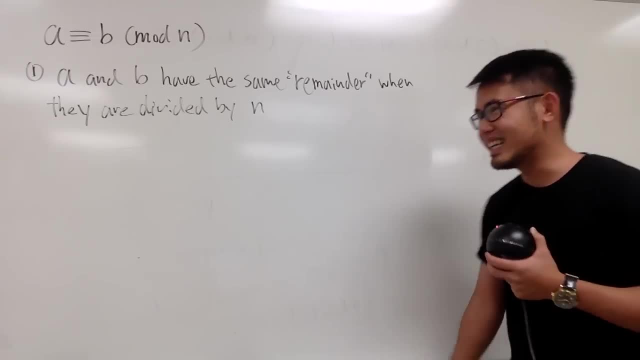 Don't do that, okay. You are pretty much just killing all the math, killing all the numbers you read, so don't do that, Okay. so this is the first way to interpret this. notation a and b have the same remainder. 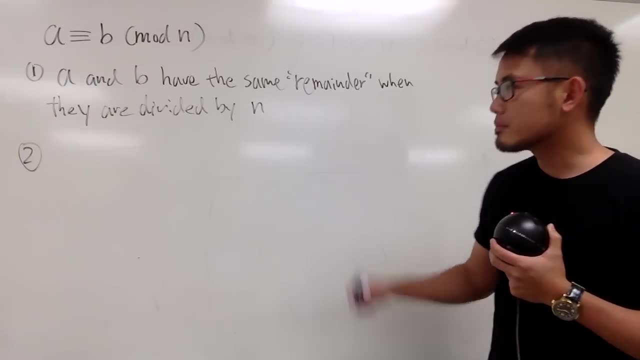 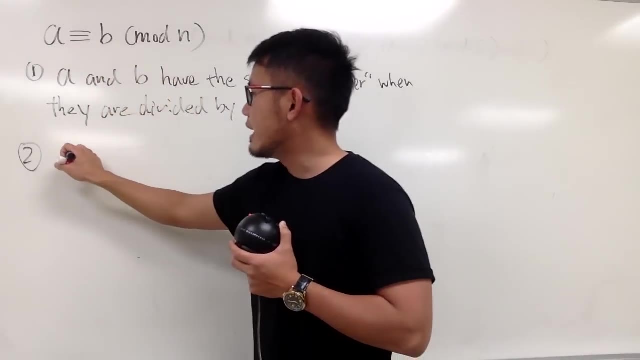 when we divide a by n, when we divide b by n. So that's the first thing. The second thing is that I can write the following: When we have a is congruent to b mod n, we can say: a is equal to. 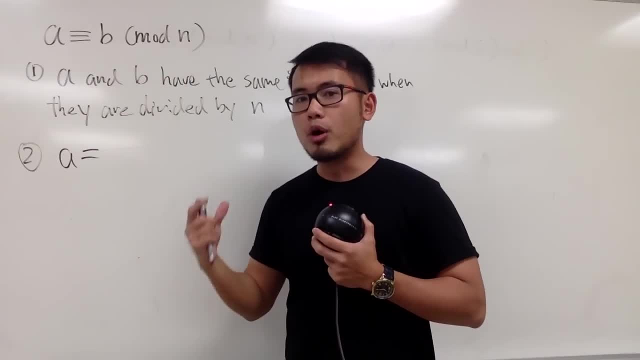 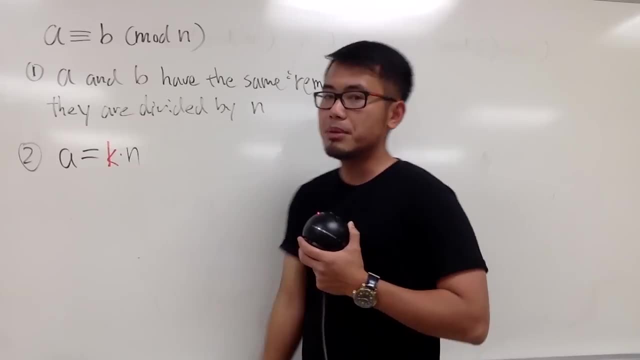 well, it's just going to be off by a multiple of n, and usually we can just say k times n for some number k which we don't know yet. just keep it as how it is for now, And then you add b to it. 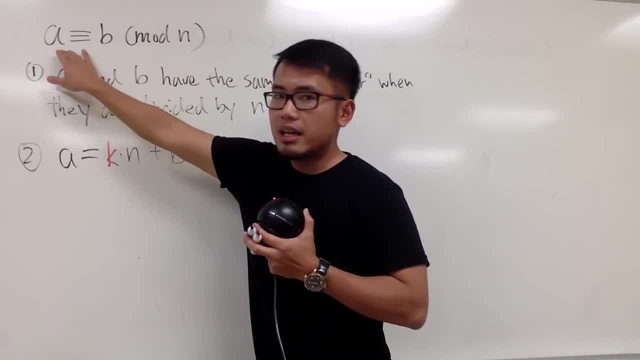 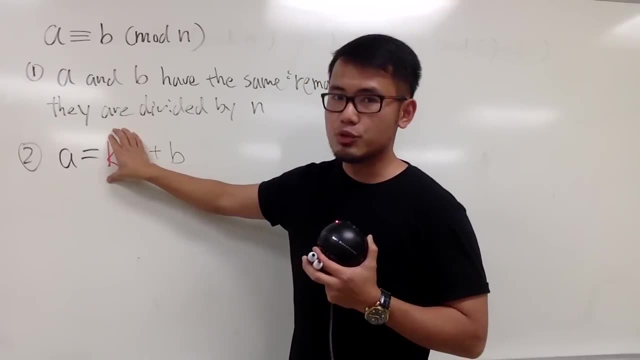 And you see, when you mod n, this right here states as a. When you have k times n mod n, this is always going to be a multiple n, so it becomes 0 in the mod n world, and then you're left with the b right here. okay. 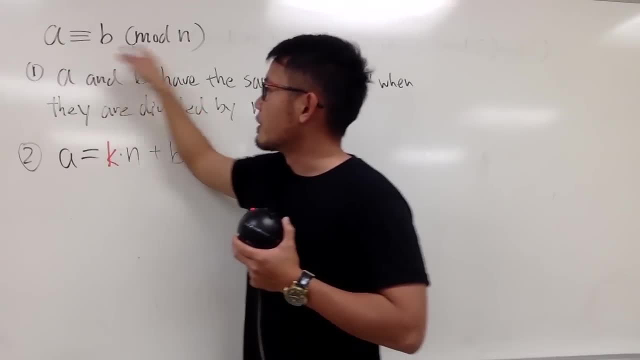 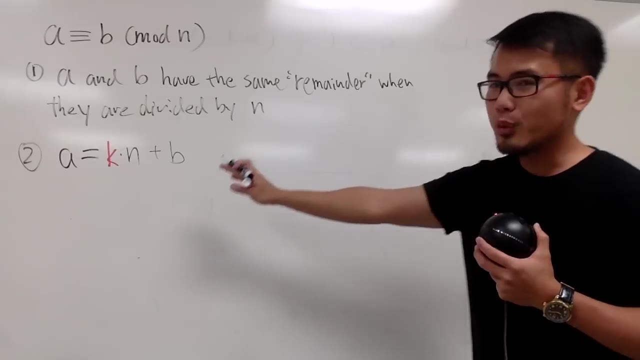 So sometimes it may be helpful when you go from here to here, because from here you're working with an equation rather than a congruence. So that's another way to use this notation. I would say another way to interpret, another way to approach when you have a congruence. 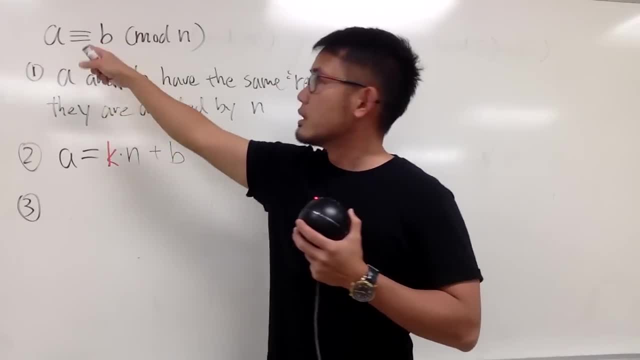 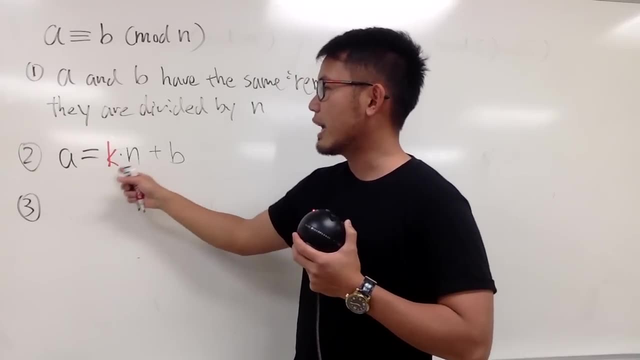 The next thing is that, okay, I can just subtract b on both sides, right? And if you subtract b on both sides, you can see that a minus b is equal to k times n. In other words, a minus b is a multiple of n, right. 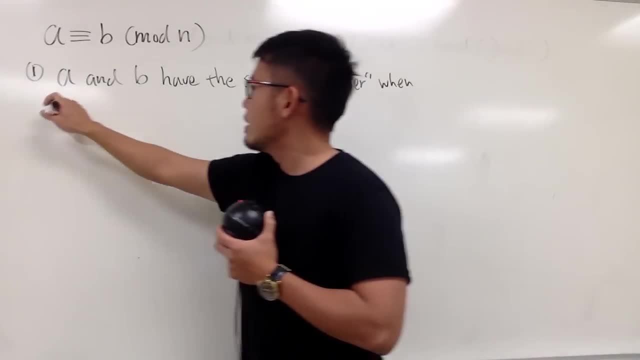 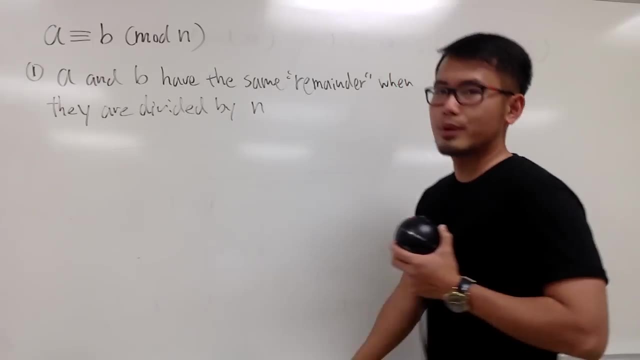 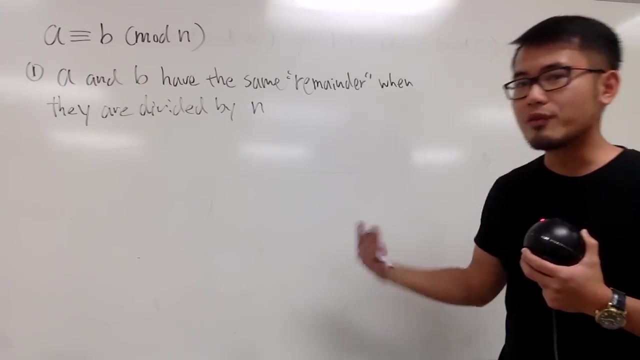 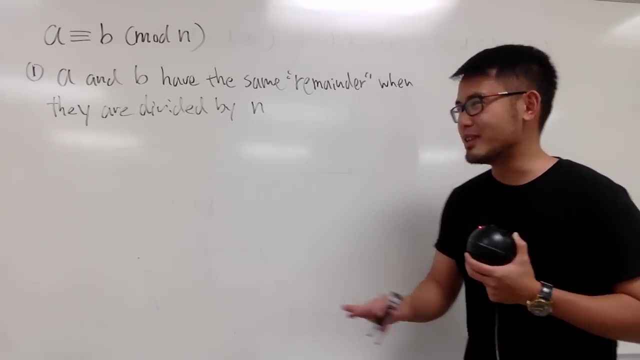 the same remainder when they are divided by n. okay, and by the way, n shall be a positive whole number greater than one. so two, three, four, five and so on. do not ever say an n is equal to 1, mod 1 kills everything. Don't do that, okay. 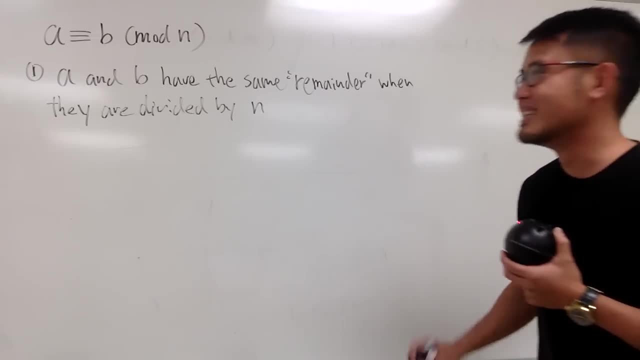 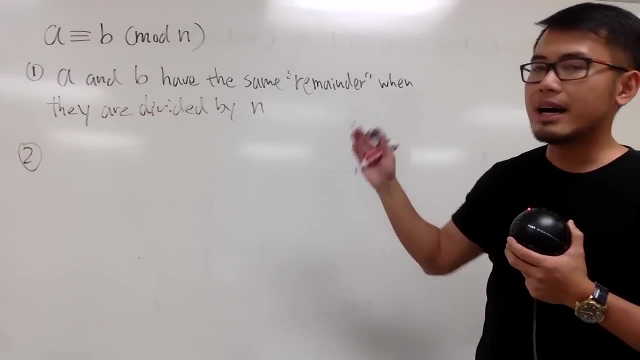 You are pretty much just killing all the math, killing all the numbers you read, so don't do that, Okay, so this is the first way to interpret this notation: a and b have the same remainder when we divide a by n, when we divide b by n. 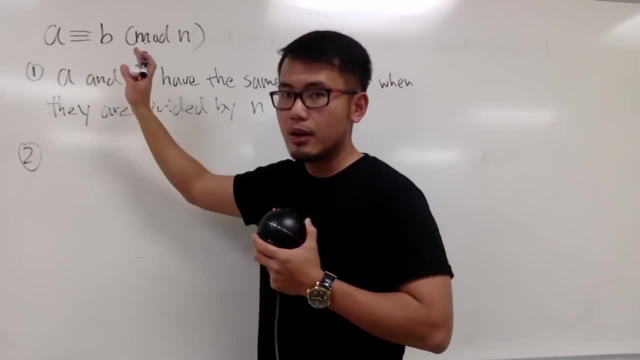 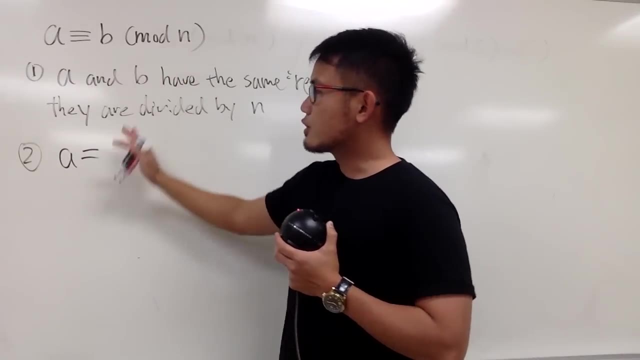 So that's the first thing. The second thing is that I can write the following: When we have a is congruent to b mod n, we can say: a is equal to well, it's just going to be off by a multiple of n. 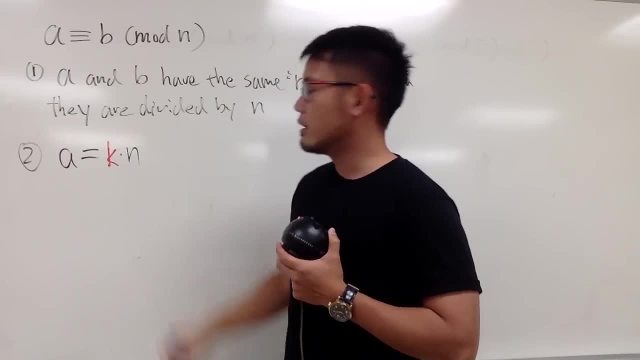 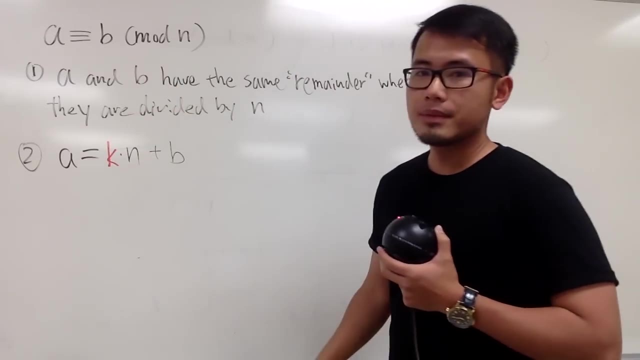 and usually we can just say k times n for some number k, which we don't know yet. just keep it as how it is for now, And then you add b to it And you see, when you mod n, this right here states as a: 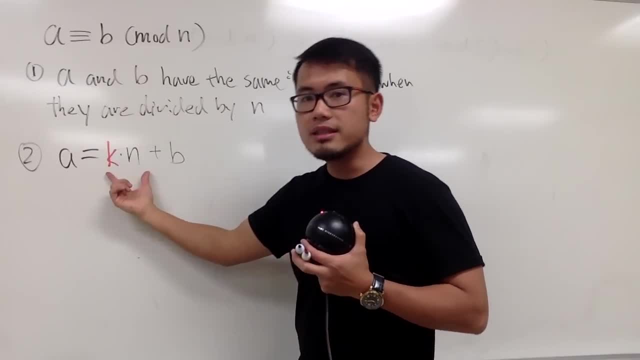 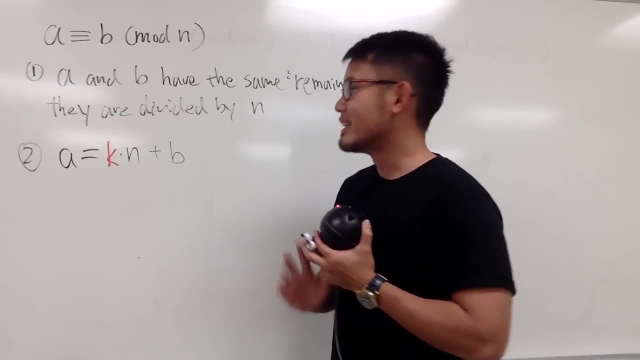 When you have k times n mod n, this is always going to be a multiple n, so it becomes 0 in the mod n world, and then you're left with the b right here. okay, So sometimes it may be helpful when you go from here to here. 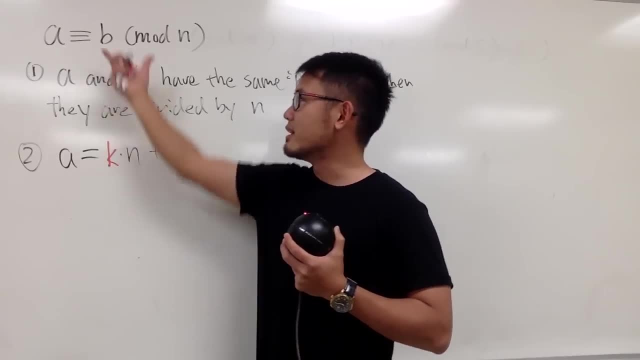 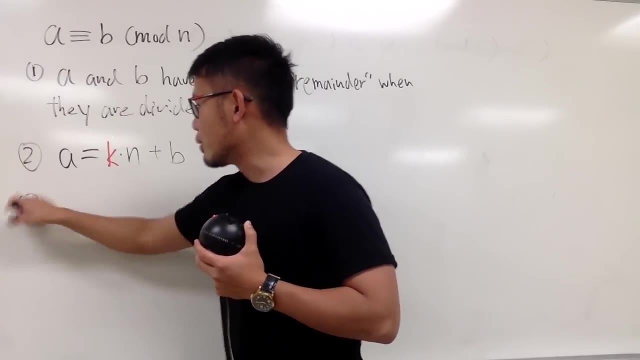 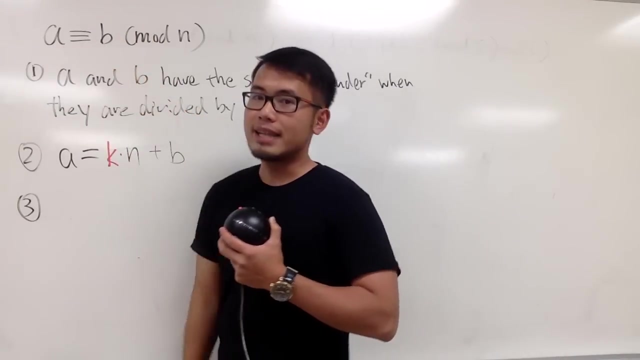 because from here you're working with an equation rather than a congruence. So that's another way to use this notation. I would say another way to interpret, another way to approach. when you have a congruence, The next thing is that, okay, I can just subtract b on both sides, right? 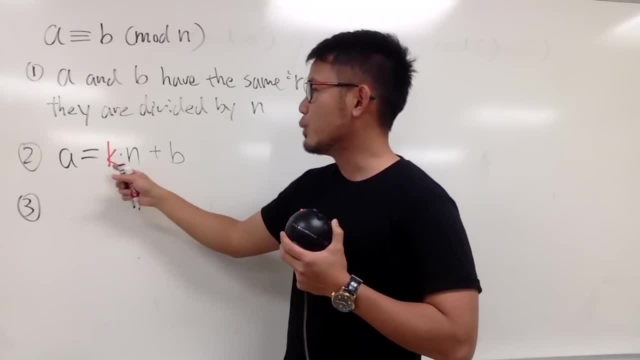 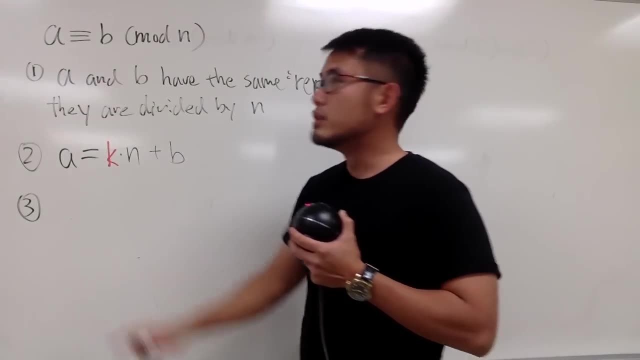 And if you subtract b on both sides, you can see that a minus b is equal to k times n. In other words, a minus b is a multiple of n, right? So I can actually go from here and tell you guys that. 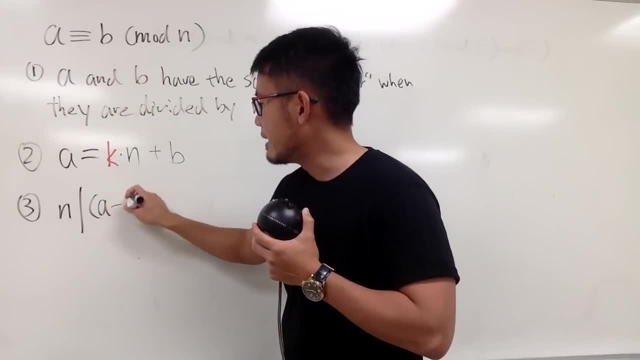 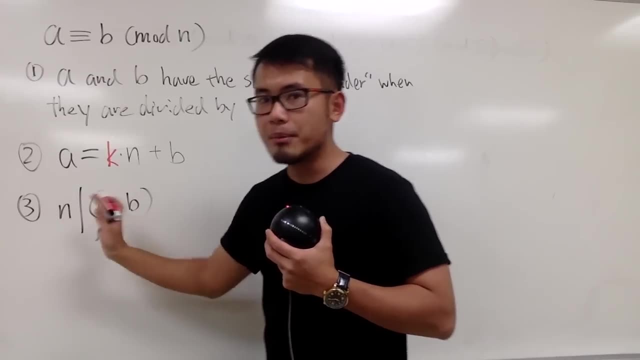 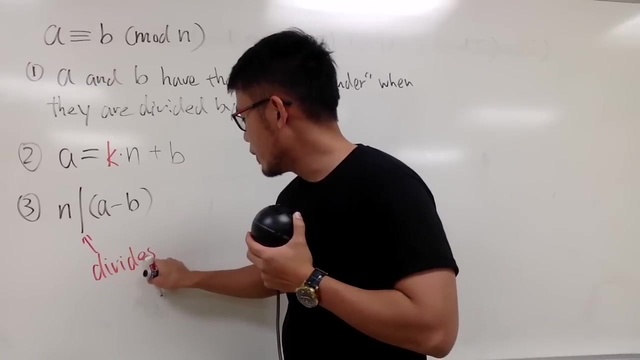 n divides into a minus b And once again, this right here has a few ways to interpret it. This is actually the common notation that we'll be using quite often. This right here you say that divides okay, And when we write this down, this means: 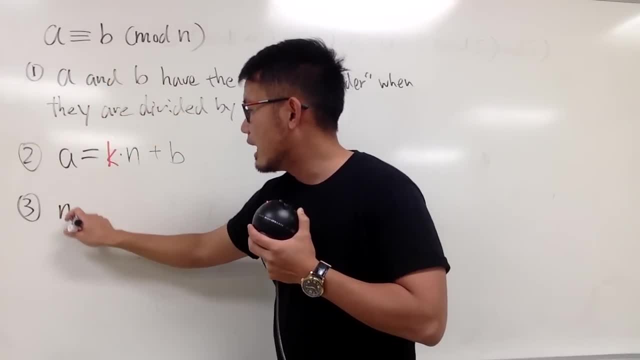 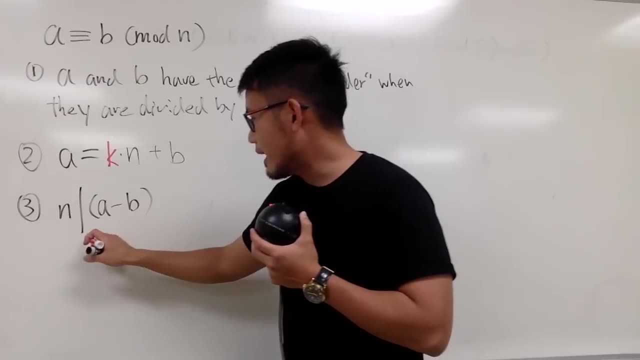 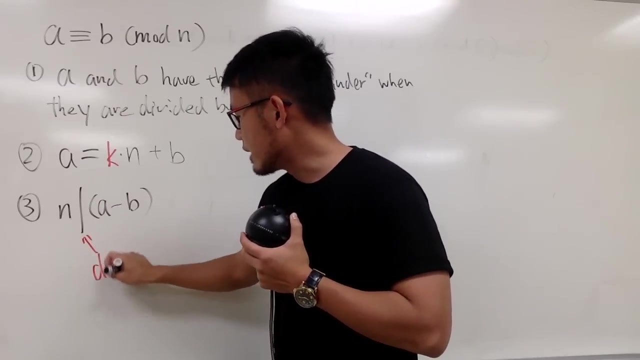 So I can actually go from here and tell you guys that n divides into a minus b And once again, this right here has a few ways to interpret it. This is actually the common notation that we'll be using quite often. This right here. you say that divides, okay. 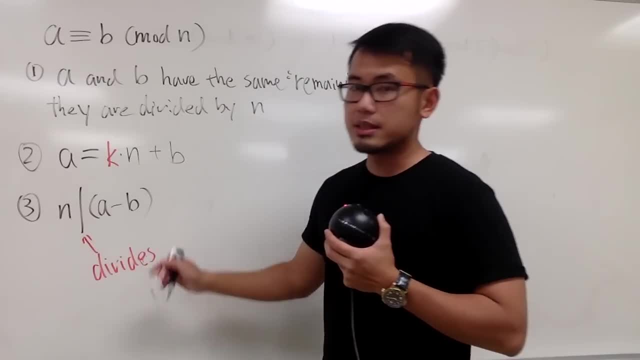 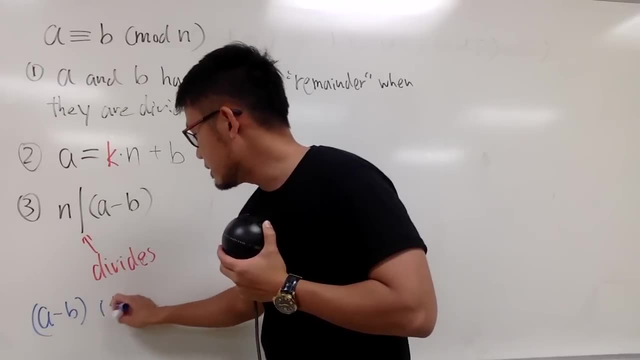 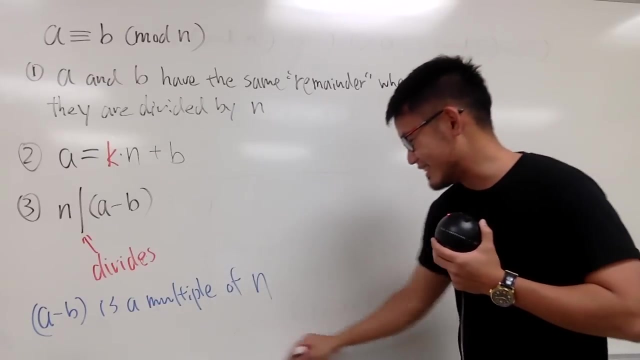 And when we write this down, this means, let's put this down in blue, like: why not? This means that a minus b is a multiple of n. okay, So that's the idea. So that's pretty much it, right. 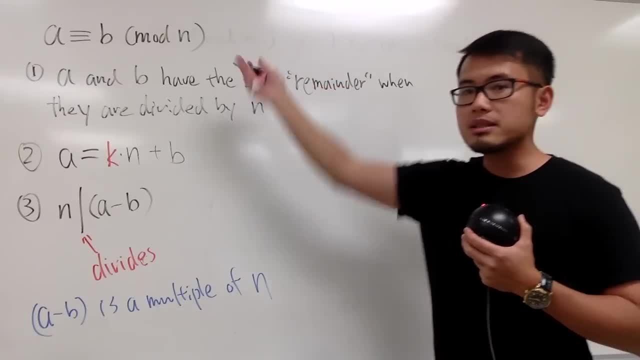 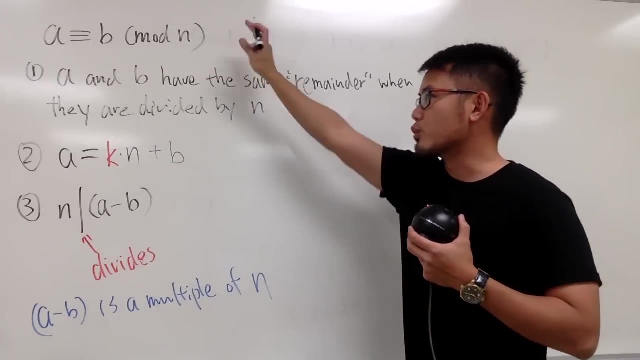 I think this is just perhaps the most natural way to know what that means, And this right here is pretty useful when you're trying to solve one equation from a congruence right. You change your congruence to an equation first, And then this right here. 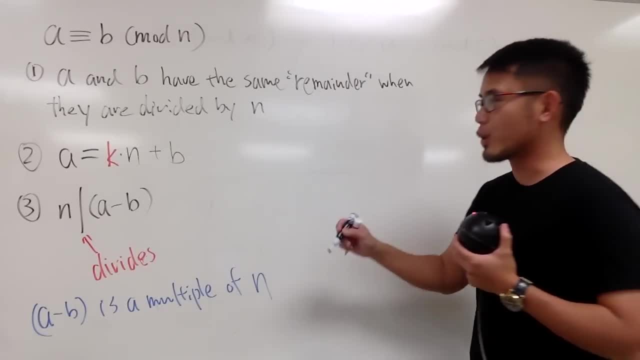 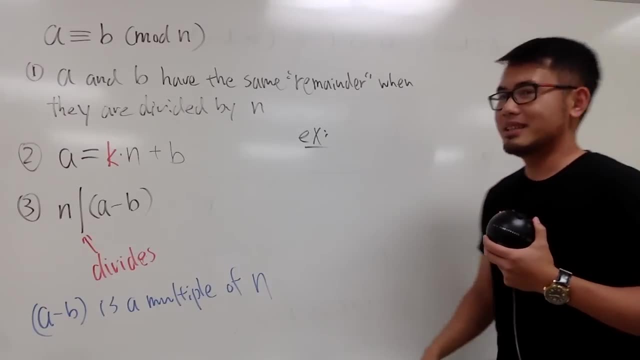 is useful when you're doing some proofs And perhaps I will just give you guys a quick example, okay, So this is just a quick example. So let's do an easy one. I would say: Let's say we have 10, okay, 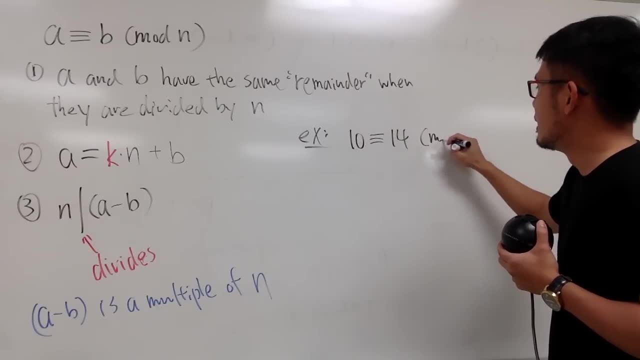 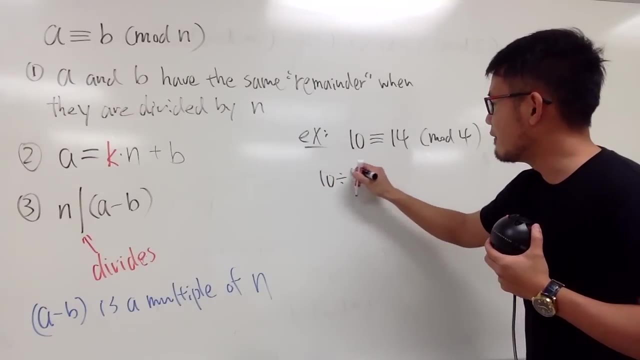 And that's congruent to 14. Math 4. Is it? Yes, it is Why? Because when you have 10 divided by 4, this right here gives you 2, with the remainder 2, right. So this right here. 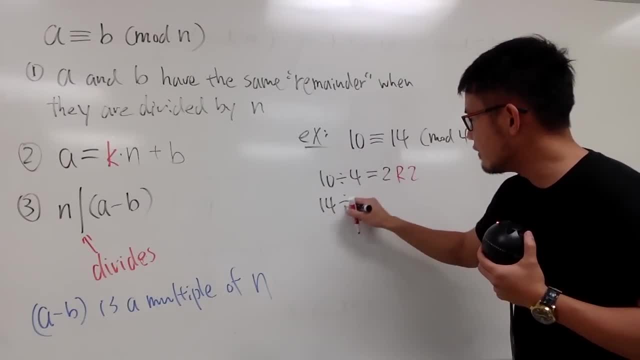 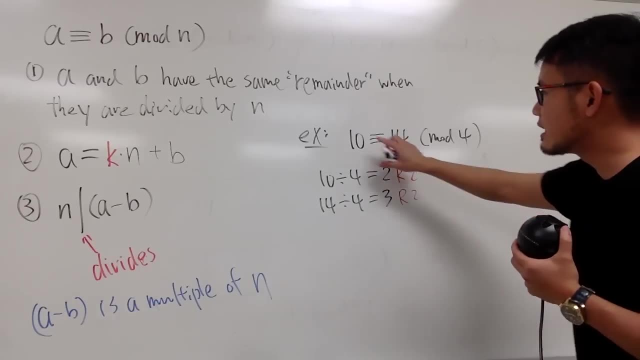 is pretty much 2.. And then right here, when you do 14 divided by 4, you get 3 with the remainder 2 as well. So they have the same remainder And once again, sometimes you may be dealing with negative number. 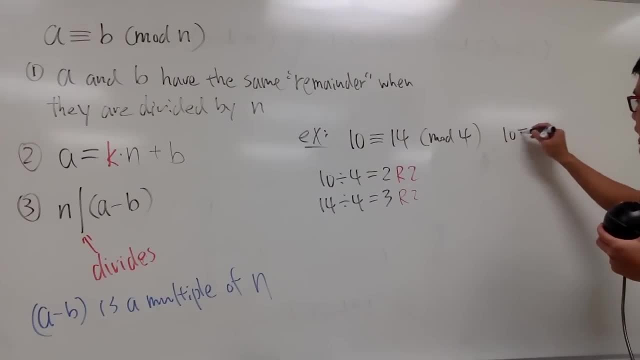 And I can also tell you guys that 10 is congruent to negative 2.. Math 4, okay, And this is 2 on the left-hand side, This is negative 2.. But the truth is that you can just go from negative 2 and you add 4 to it. 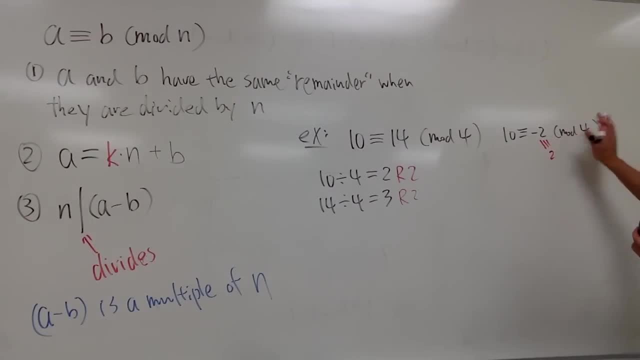 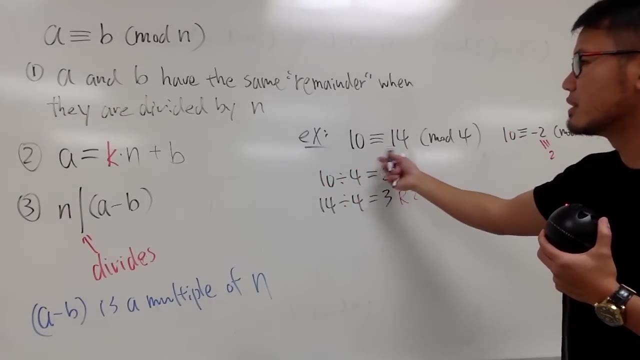 Negative: 2 plus 4, this is also the same as 2, Math 4,. okay, So that's the idea. Now the second thing is perhaps slightly trickier, because I told you guys, we have this huh. 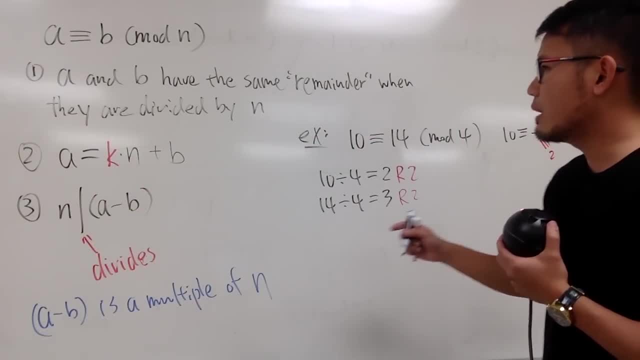 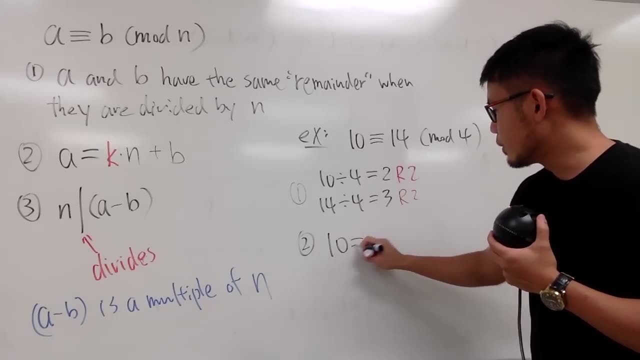 And I want to write this down. Okay, A is my 10 right here, based on the order, and this is the first way. The second thing is that I will write: 10 is equal to k- I don't know yet- multiplied by 4.. 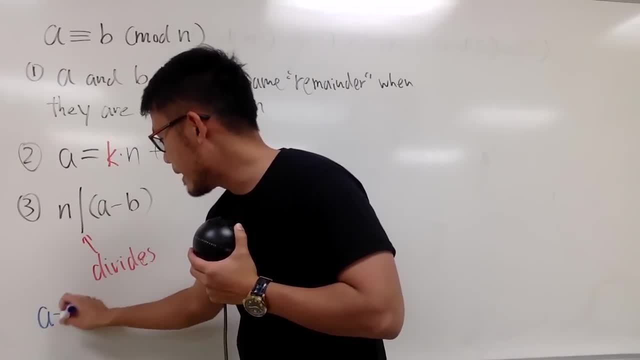 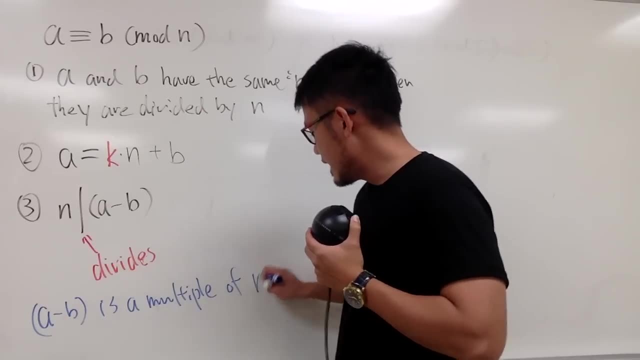 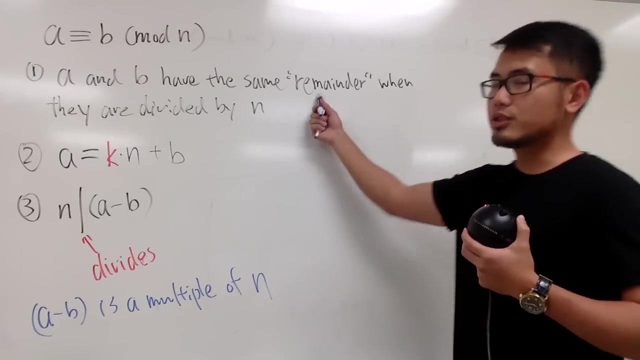 let's put this down in blue, like: why not? This means that a minus b is a multiple of n. okay, So that's the idea. So that's pretty much it, right? I think this is just perhaps the most natural way to know what that means. 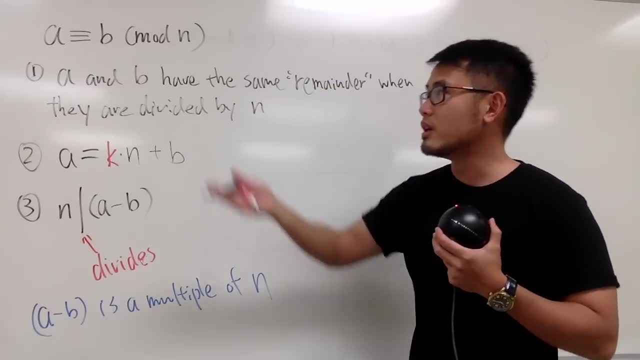 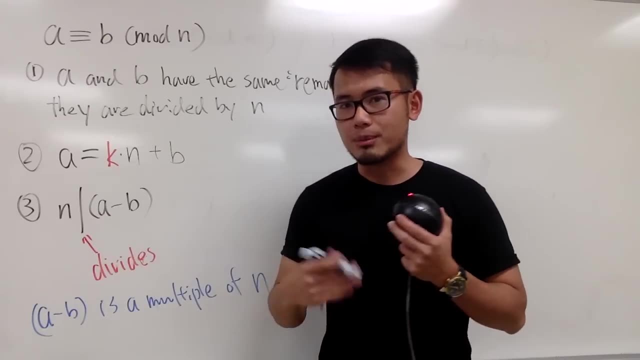 And this right here is pretty useful when you're trying to solve for an equation from a congruence right. You change your congruence to an equation first And then. this right here is useful when you're doing some proofs, And perhaps I will just give you guys a quick example. okay, 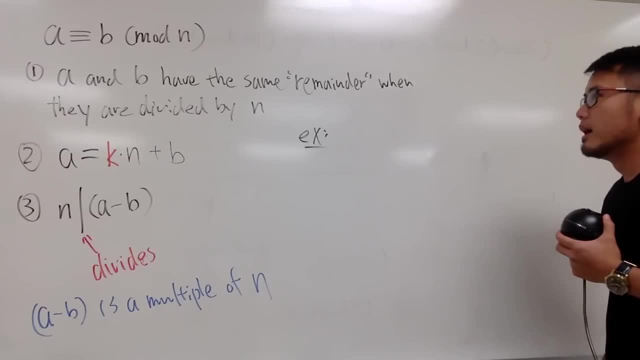 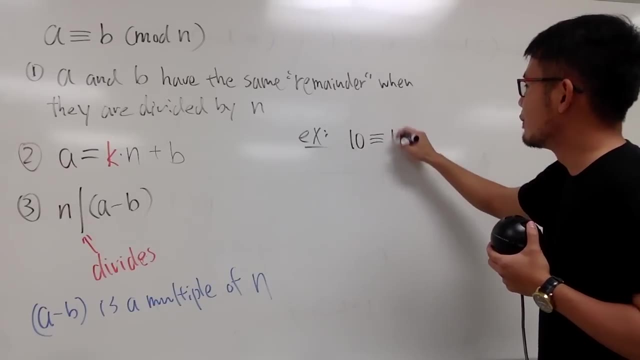 So this is just a quick example, So let's do an easy one. I would say: Let's say we have 10, okay, And that's congruent to 14. Math 4. Is it? Yes, it is. 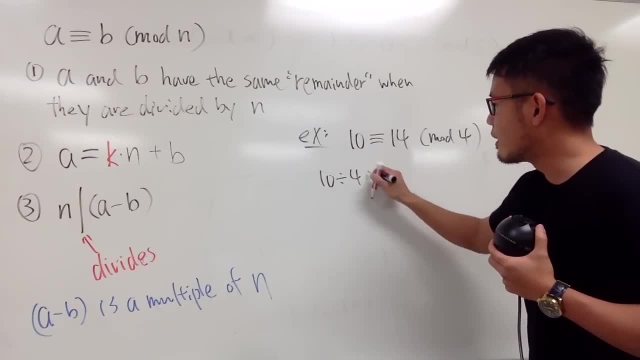 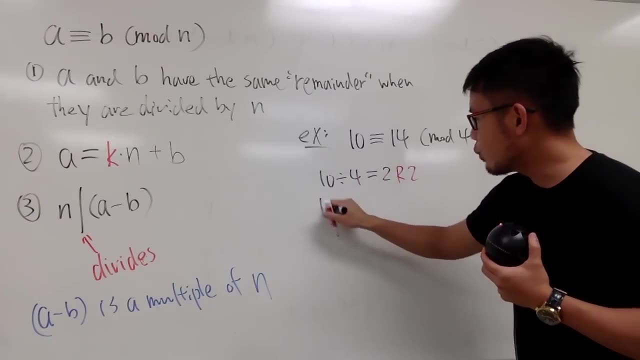 Why? Because when you have 10 divided by 4, this right here gives you 2, with the remainder 2, right. So this right here is pretty much 2.. And then, right here, when you do 14 divided by 4,. 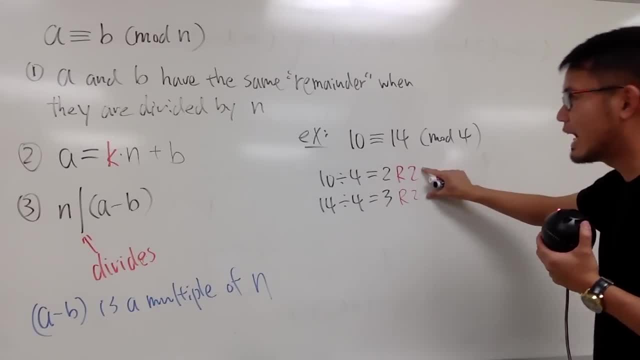 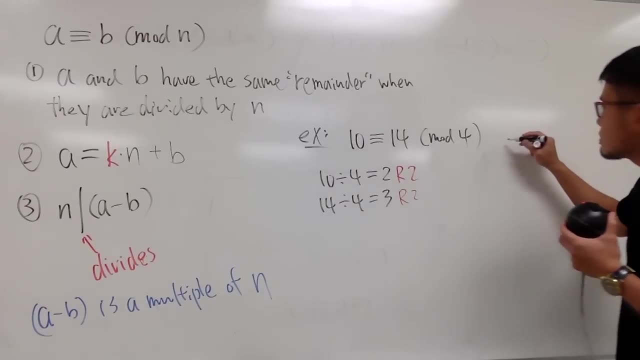 you get 3 with the remainder 2 as well, So they have the same remainder And once again, sometimes you may be dealing with negative number And I can also tell you, guys, that 10 is congruent to negative 2.. 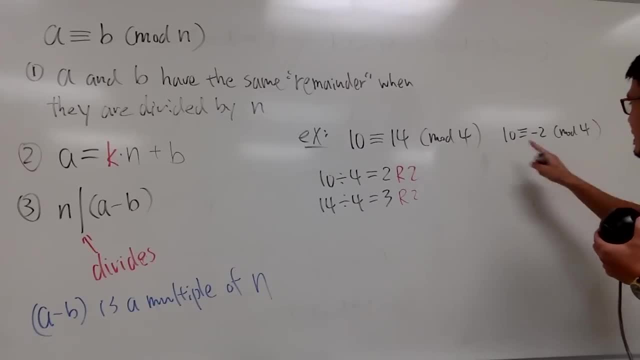 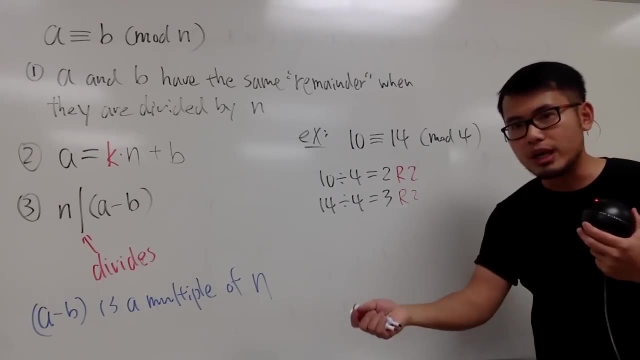 Math 4, okay, And this is 2. on the left-hand side, This is negative 2.. But the truth is that you can just go from negative 2, and you add 4 to it. Negative 2 plus 4, this is also the same as 2.. 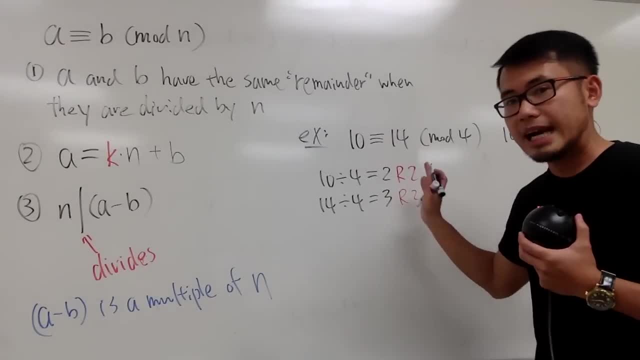 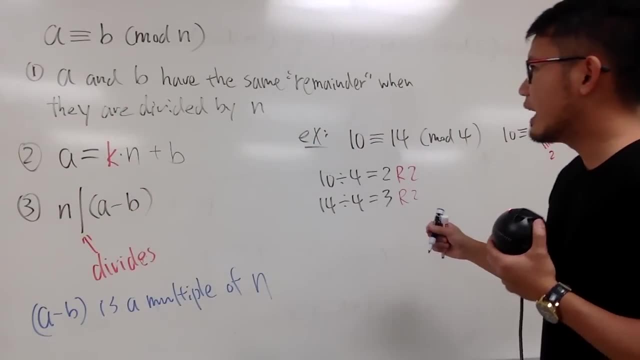 Math 4, okay, So that's the idea. Now the second thing is perhaps slightly trickier, because I told you guys, we have this huh And I want to write this down. Okay, A is my 10 right here, based on the ordering. 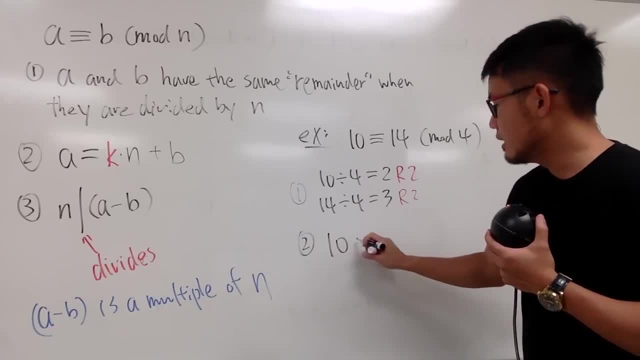 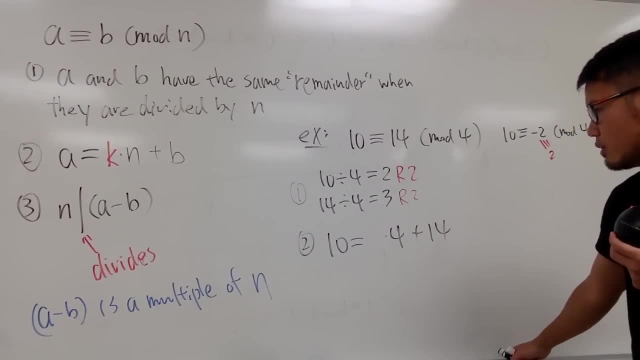